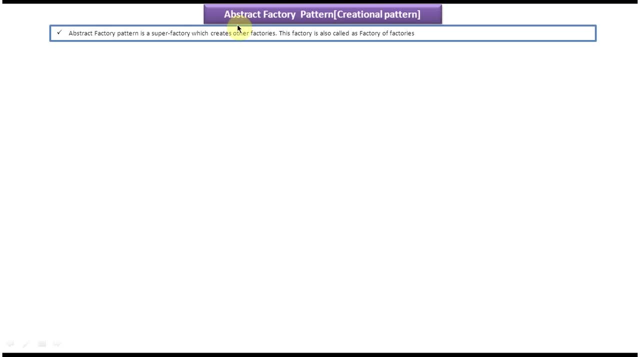 Hi, this video tutorial I will cover abstract factory design pattern. Before you watch this video tutorial, please login to my channel and watch: factory design pattern: introduction. factory design pattern- implementation. factory design pattern, class diagram and sequence diagram video tutorial. Then come and watch this abstract factory design pattern so that they will 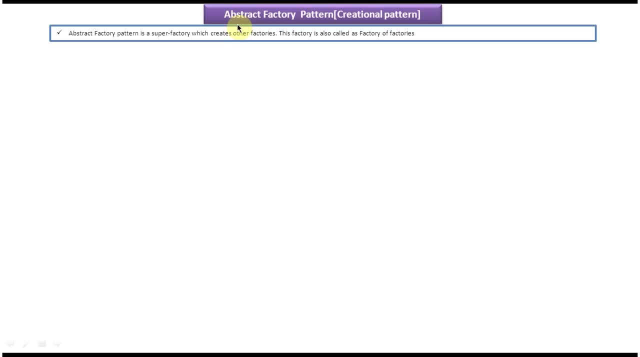 understand this abstract factory design pattern very clearly. This abstract factory design pattern falls under the category of creational pattern. First we will see the explanation of abstract factory design pattern. This is the explanation I will just read out. Abstract factory pattern is a super. 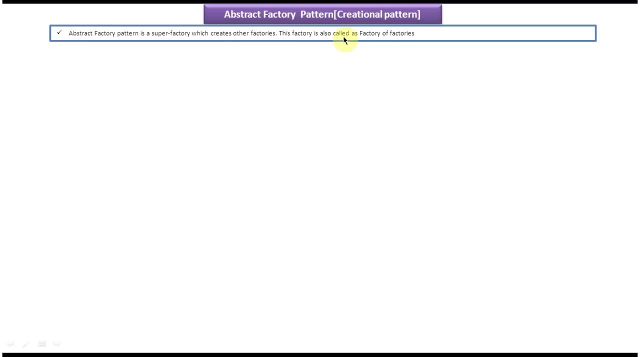 factory which creates other factories. This factory is also called as factory of factories. Okay, to understand this explanation, I have created one example. Okay, so here you can see cat, dog and lion. Okay, this cat class, dog class and lion class are the subclasses of animal. 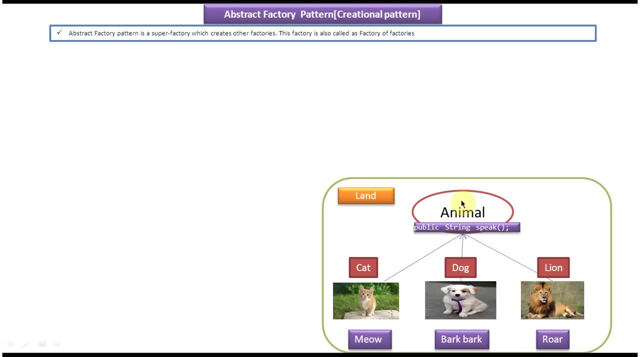 superinterface or animal superclass. Okay, this animal superinterface or superclass is one method called public string speak method and this cat will implement this public string speak method and it will return meow Like that. this dog will implement this speak method and it will return bark, bark Like. 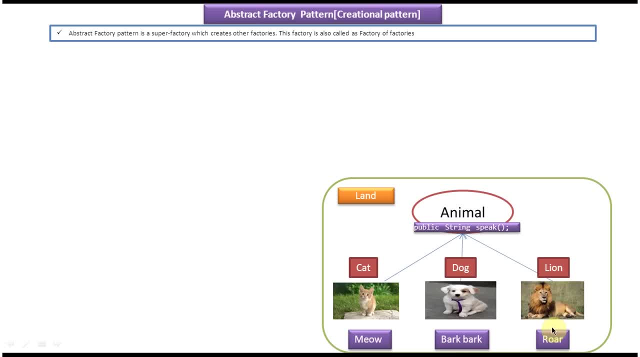 that this lion will implement this speak method and it will return roar. Okay, and this cat, dog and lion are living in the land. Okay, so that, so this, all the animals will fall under the category of land animals. Okay, so, as per the factory, 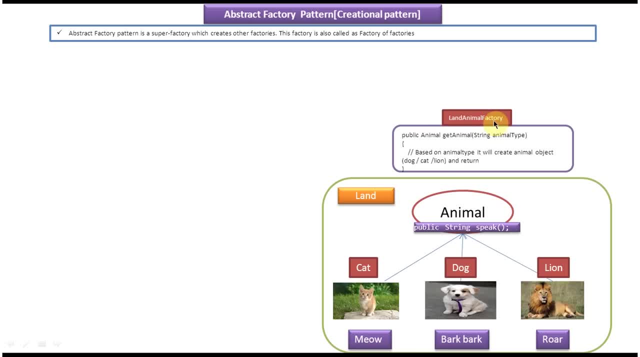 design pattern. I have created land animal factory class and as per factory design pattern we have to write a one method called get animal and the parameter should be animal type. so, based on the animal type passed, this method will create the animal object and it will return the animal object to the caller, so the animal object can be dog. 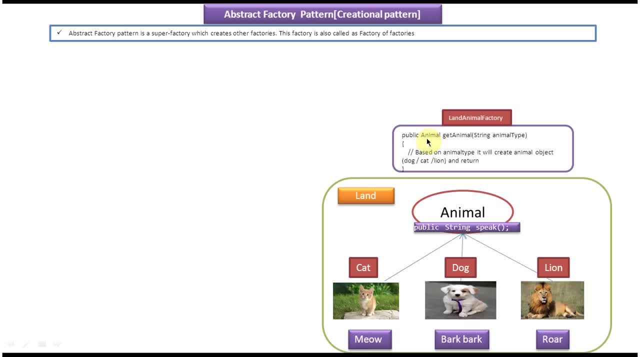 or cat or lion, okay, and this method will return superclass or super interface reference. so in this case it will return animal superclass or super interface reference. suppose, say, if we pass animal type as dog, what this method will do is it will create dog object and it will assign to the superclass or super. 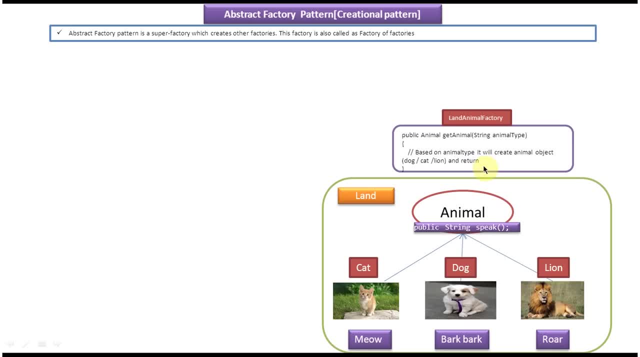 interface animal reference variable and that reference variable will be returned back to the caller. suppose, say, if if we pass animal type as lion, this method will create the lion object and assign the lion object to the super interface or superclass animal reference variable and that animal reference variable will be returned to the caller. so here in the 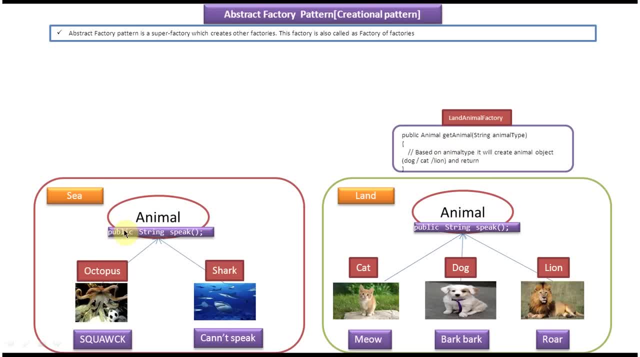 left side you can see animal superclass or super interface. it has public string speak method and you can see there are two subclasses: one is October, another one is shark, and this October's will implement the speak method and it will return squawk like that. the shark will implement the speak method and it 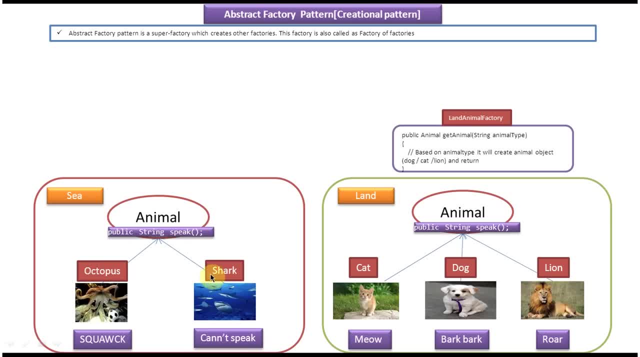 will return, cannot speak. so this October's and sharks are living in sea, so this falls under the category of sea animal. so as per factory design button have created sea animal factoring and as per factory design button, it should have one method called get animal and it should return superclass or super. 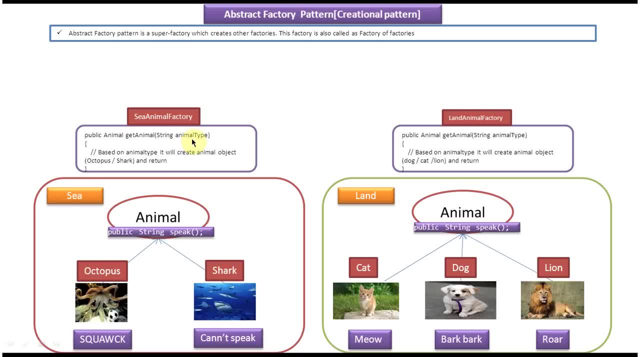 interface reference and it has string animal type as parameter. suppose if we pass October's as animal type, then what this method will do is it will create the October's object and it will assign to the superclass or super interface reference variable animal and that super class or super interface reference will. 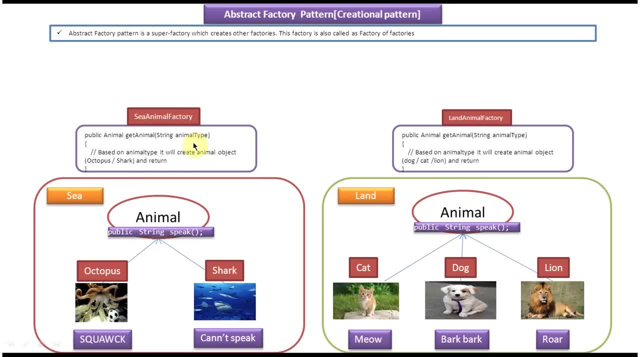 be written to the caller. so suppose if we pass animal type as shark, what this method will do is it will create the shark object and assign to superclass or super interface reference variable and that super class or super interface reference variable will return to the caller. okay, so based on the animal type. 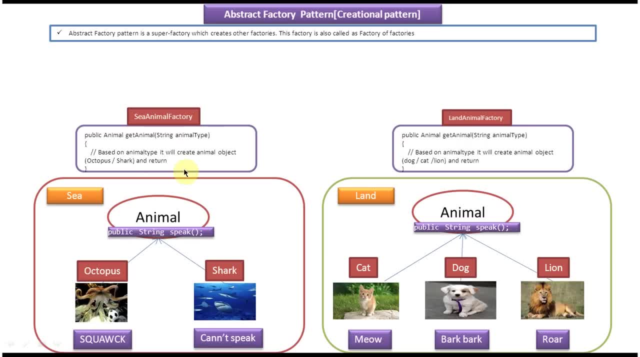 it will create the one of the animal object and it will return to the caller. so here you can see. there are two factory right here. one is the sea animal factory and another is land animal factory. so this sea animal factory and land animal factory, or subclasses of this animal, 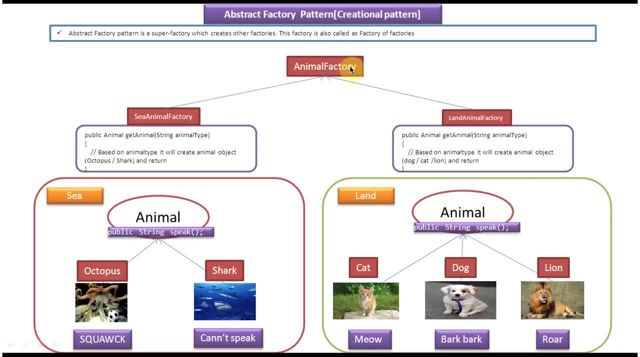 factory. okay, now we will see. what is this animal factory, what is the responsibility of this animal factory? so here, this animal factory is nothing but abstract, a factory. okay, So this animal factory is responsible for creating other factory, right? So in this case, this animal factory is responsible for creating sea animal factory or land animal factory. 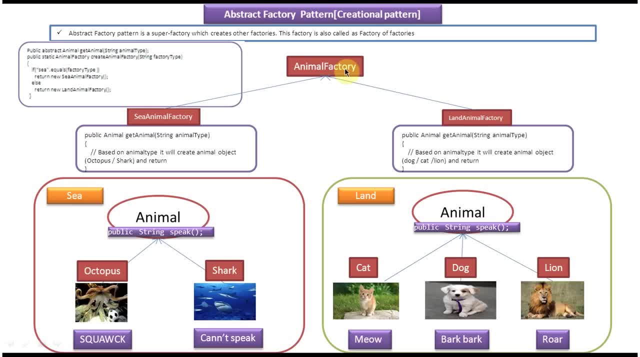 So this animal factory is called super factory. okay, So it has two methods. The first method is abstract method, getAnimal- right, So that getAnimal method is implemented by sea animal factory and land animal factory that you can see here. okay, 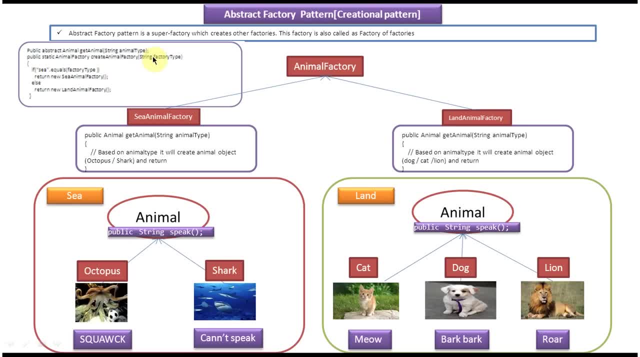 And the second method is createAnimalFactory. okay, So what this method does is based on the factory type we passed. it will create either sea animal factory or land animal factory and it will return to the caller. So, basically, this animal factory is called. 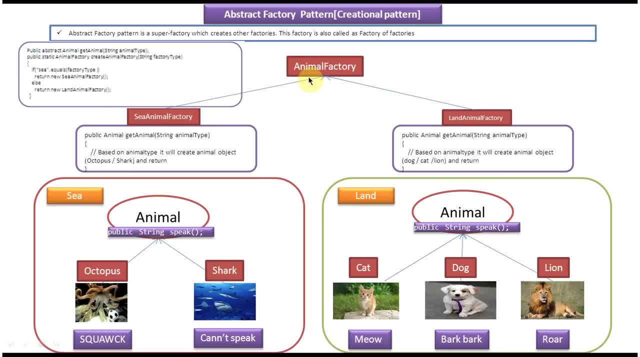 Abstract factory and it act as a super factory for sea animal factory and land animal factory and this animal factory is responsible for creating the factory classes, creating the factory objects. like it can be a sea animal factory object or it can be a land animal factory object. 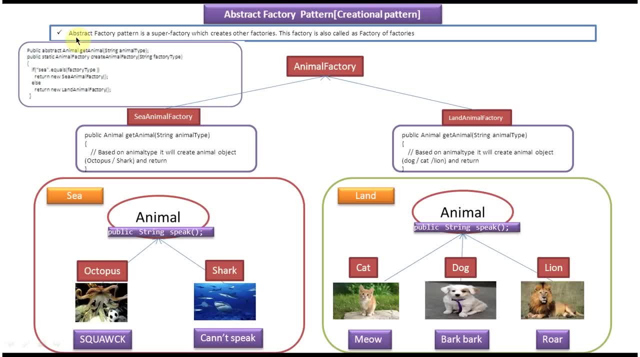 So now, if you read this sentence, you will understand clearly. Abstract factory pattern is a super factory. So in this case, This is the super factory- okay, Which creates other factories. okay, So this factory is responsible for creating other objects. 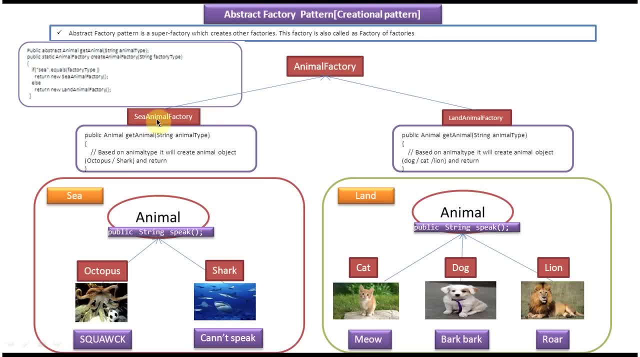 In this case, this animal factory is responsible for creating sea animal factory or land animal factory, based on the parameter we passed right here, And this factory is also called as factory of factories Because it is a super factory, So it is called factory of factories, okay.